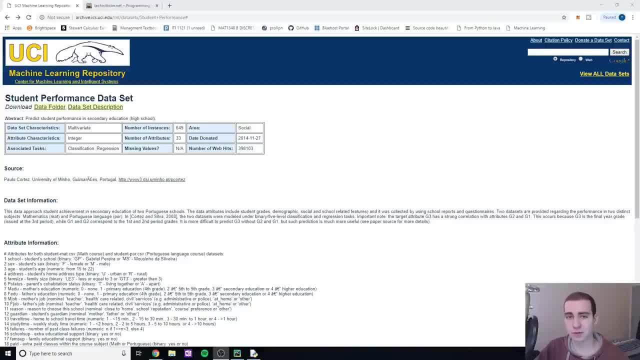 Hello everyone and welcome to kind of the first official machine learning tutorial. We're actually going to be writing code and reading in data. So in this video, essentially we're going to be getting a big data set and we're going to be minimizing that data set to use the valuable information out of it. which is very important and is honestly probably the hardest thing with machine learning is getting your data in the right form and using proper and valid data. And then we're going to be actually in the next video, implementing it's called the linear regression algorithm. 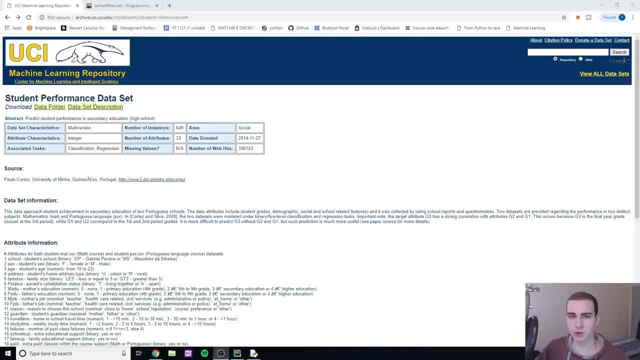 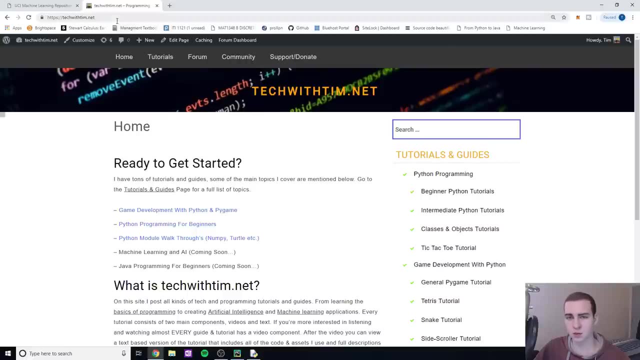 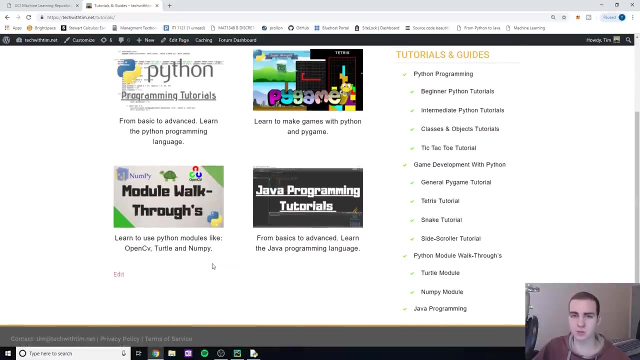 To predict grades based on kind of student behavior and student past grades. So that's a data set we're going to be using. It's actually what I have open here, which I'm going to talk about in just a second. But before I move into all of that, I just want to say that if you'd like to follow along with the tutorials and see all of the code, have all of the data, go to my website, techwithtimnet. If you go to the tutorials page here, you will see- I know you don't see it right now, but there'll be a little box here that says machine learning with Python And if you click on that you'll find the tutorial series and you could go through and 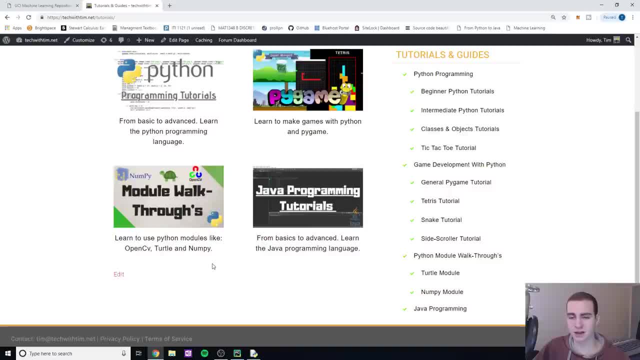 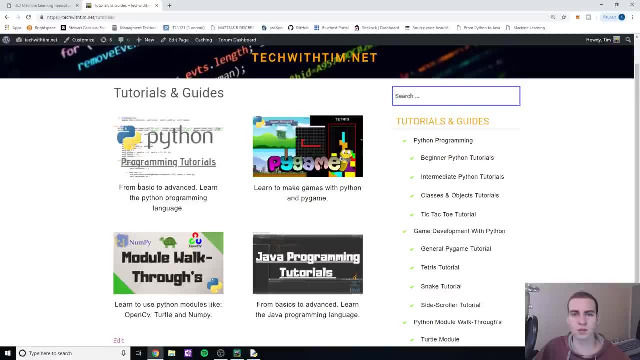 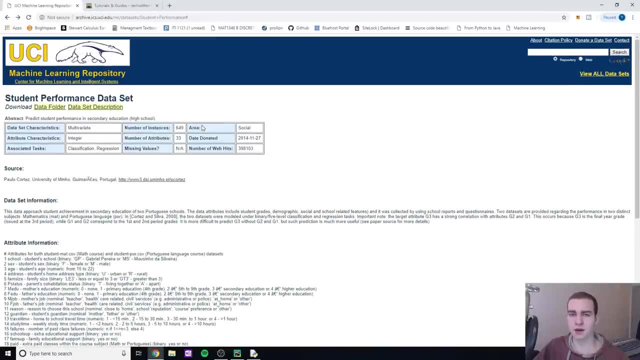 it's going to have all the code, all of the data, everything that I write and kind of some descriptions as well. It's not going to be as extensive as the video, But just in case you want to get all the code and stuff, it'll be on the website. So I recommend that you follow along with that, And that's going to be for the future of all of these machine learning videos as well. Okay, so back to our data Now. with machine learning, data is obviously the most important part by far. Now, the algorithm is actually fairly easy to implement, but we have to implement them on certain data, And our data has to be in a correct form. 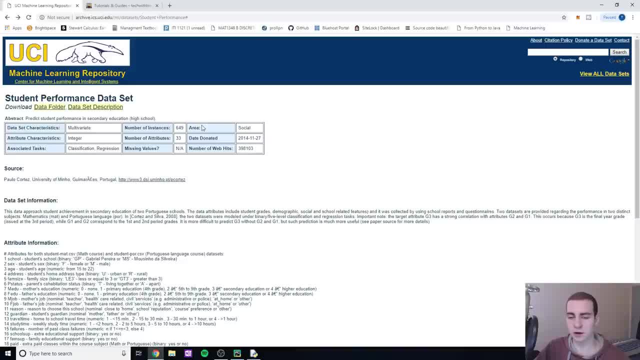 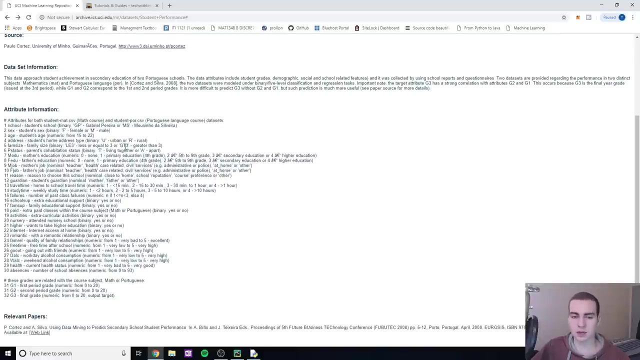 In a correct shape And it has to be well valid data like. it has to make sense, right. So essentially what I'm doing is I'm just going to download a data set off of this UCI machine learning repository website And they have a ton, ton of ton of data sets. So I just picked this one because I thought it was kind of interesting- student performance data set- And essentially you guys can read the data set information. this link will be in the description and on my website as well, And it goes through a bunch of things that I want to walk through them with you so that if you want to pick your own data sets off the website, you kind of 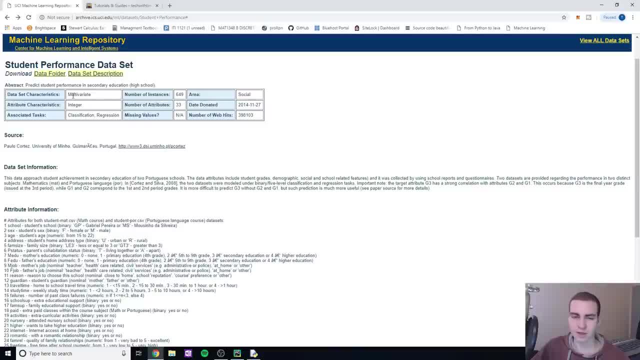 know how to do that And what all these different things mean. So probably some of the more important things I guess. actually I'm just gonna read through them all And I guess I'll talk about them as we go. So data set characteristics here and it'll show you these all on the main page when you select data sets as well. Multivariative just means it has, I believe, more than two variables, So you don't just have like one variable corresponding to the other one. there's a ton of different attributes that will apply to a certain label or classification characteristics. don't worry about that attribute characteristics. 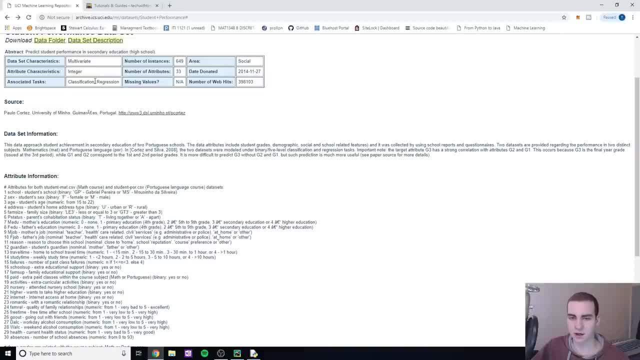 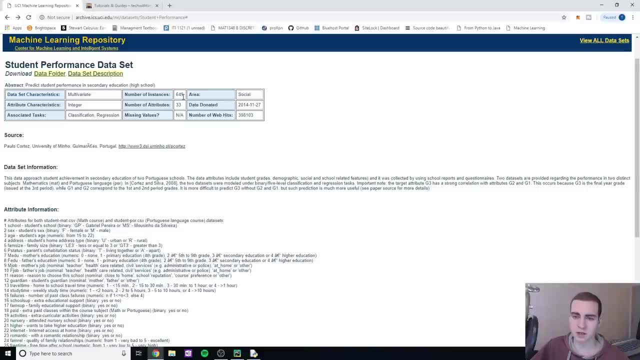 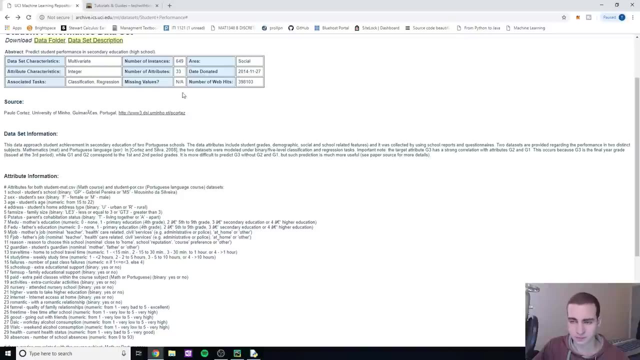 That's actually incorrect. But associated tasks, classification, regression. this is just what it's good for Typically. you can obviously use this data set with other kind of algorithms, but that's what it recommend is. number of instances is how many instances are like people are in this case, students are actually in the data set. Number of attributes is how many attributes for every single instance? Okay, quick side note: if you guys hear me like coughing or notice I'm a little bit not as good as I usually am. I am a little sick right now, So if you 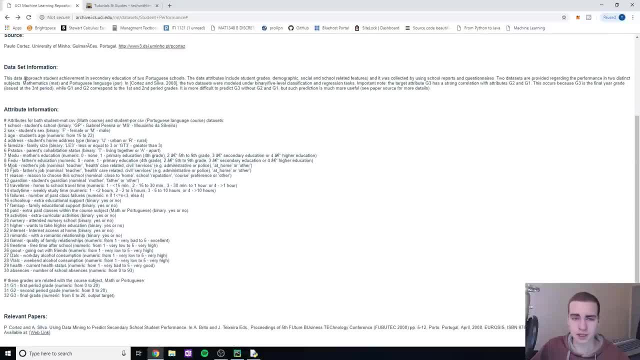 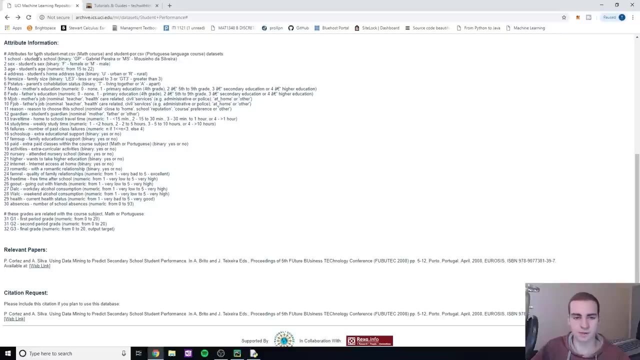 notice my voice a little raspy, please excuse me. So data set information. essentially, this is good to read, kind of tells you how they got the data, what it's from, It's not crazy important, But I mean it kind of tells you what all these attributes are meant for. And then attribute information. This is like each property of a student- right Or attribute is obviously the best way to say it- And it'll go through what the name of the attribute is and then all of the different values that can be associated with that. So for us, we're going to want to deal with integer attributes. So already, 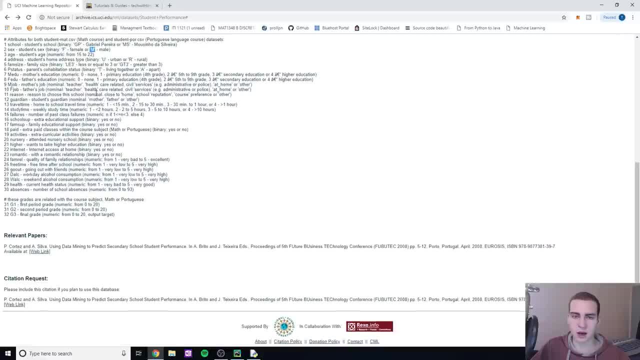 anything that says like male, female, like we don't want to use these Because unless we're going to transfer them, transfer them into like a zero or one, just gonna be more difficult later on, So like study time failures, like you can read through these and see what they all are, And each data set will have attribute information. Typically, the most important attributes for us in this data set are going to be the grades, So grade one, grade two and grade three, And pretty much we could just use these two grades to predict what a final grade would be And that would give us a fairly accurate result. 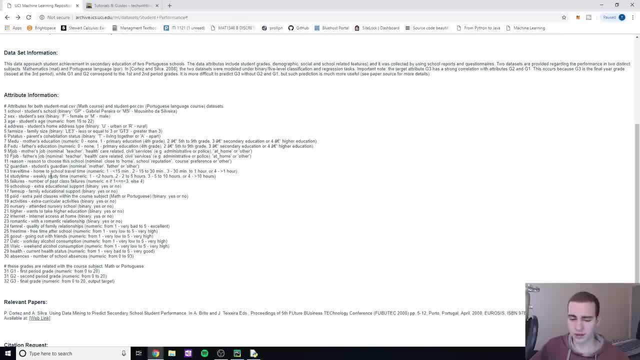 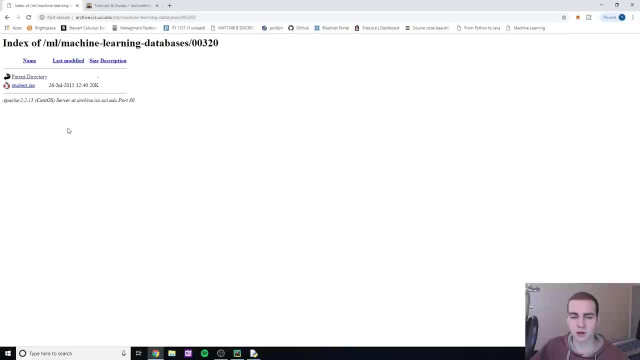 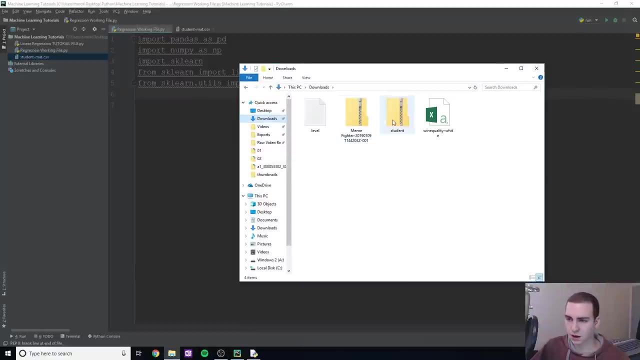 But I want to mix in some of these other attributes as well and see what we can do with them. Okay, so that's the data we're going to be using to download that. go to data folder. go to student zip. it will download the zip, for you already have a download, So I'm not going to do that. And then when you open up the zip, let's go to my downloads here. It'll look something like this: Click on student mat and then just drag that into whatever directory you're working in. Okay, because you can use this Portuguese one. it'll be the exact same process, except hyphen POR instead of mat. when you were 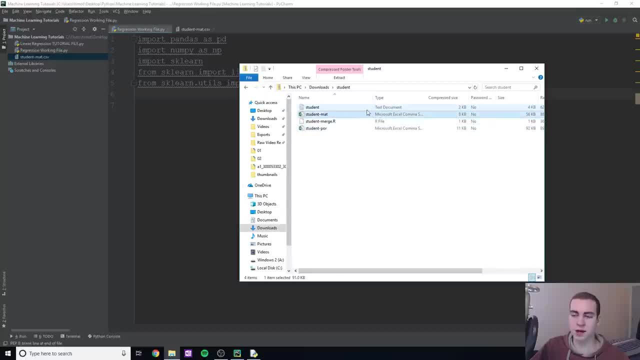 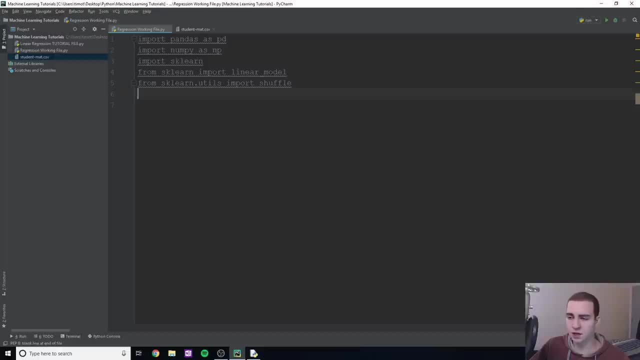 importing it, But this is just a math class to support these class. I like the math class better personally, So that's what I'm going to use. Okay, So now that we are actually we're in Python, so I'm in what you call this here, PyCharm- we're actually going to need to just set up a few things before we can actually start importing our data. So in the last tutorial I installed some packages. we need to actually install some more packages that I forgot about, So excuse me for that, But essentially we're going to activate our environment again to fresh reminder. we can just do activate. 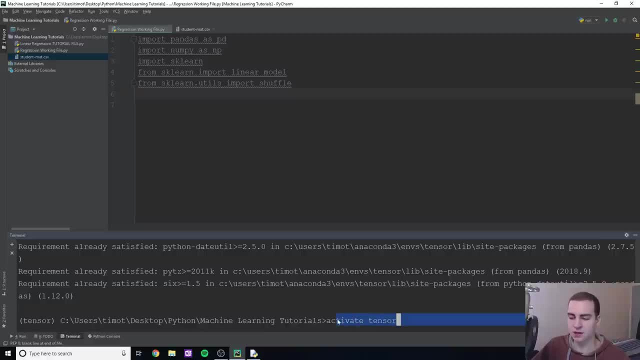 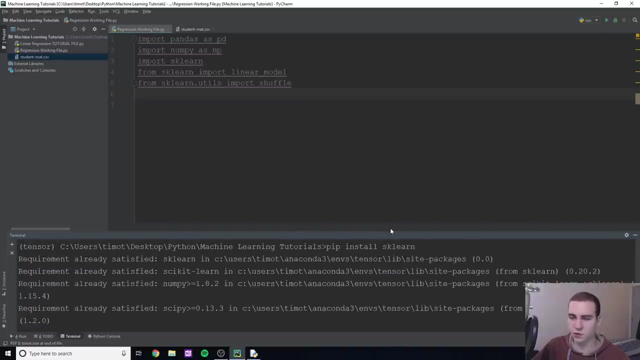 and then in my case I called mine tensor. So we're going to do that And I've already done that, you can see, I because I have tensor right here- And we're going to install some packages. So the first one we need to install is pip, install SK learn. So I already have it installed, but run through that will take a second. We also need to install NumPy and pandas, So we'll install pandas. this is going to allow us to read in our data frames really easily, Or data sets, sorry, not frames, I keep calling it frames, Anyways. 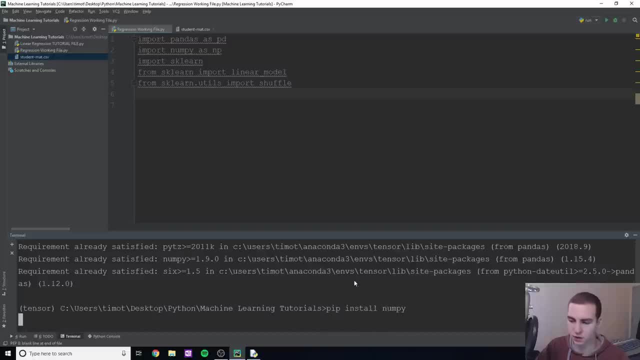 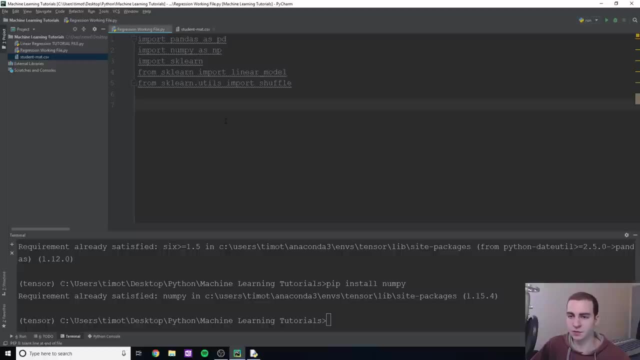 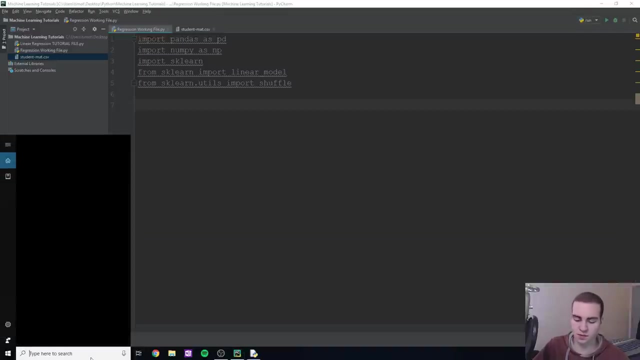 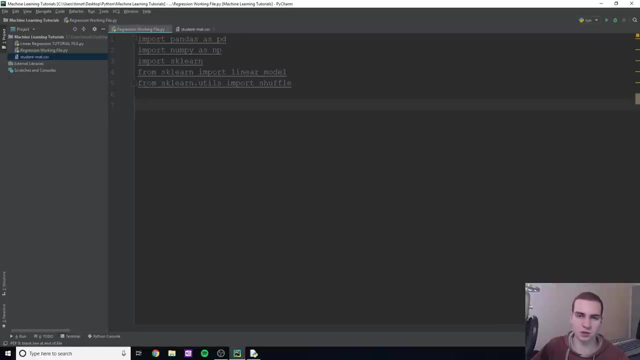 we'll do pip, install NumPy as well. This is just a allows for arrays, because all the stuff we do actually needs arrays, not lists, And Python doesn't have general support for arrays. Okay, So once we have those installed, we can close this terminal. And, by the way, you could have done this from the command prompt as well. Just by running the terminal. it just runs it in the main directory that you're already in. So I don't know, I just do that because it's easier in PyCharm. But yeah, Okay. so first thing we need to do is read in our data sets. you can see already have my 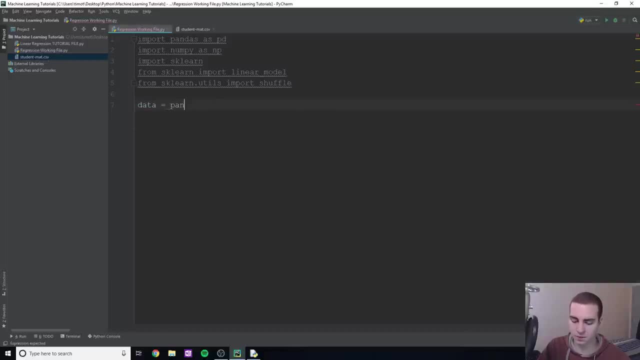 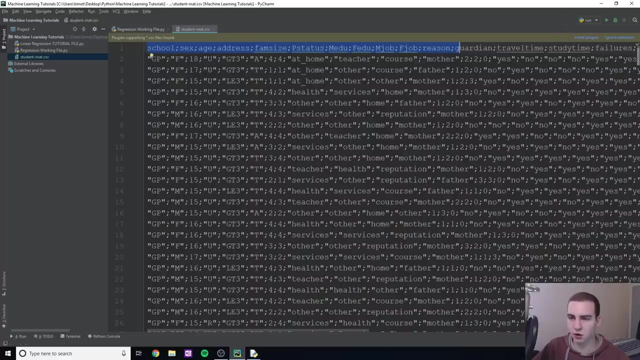 here. So do this. we're going to say: data equals pandas And I think I actually brought that in as PD. So just copies import statements here. pd dot read CSV. And of course that didn't work. Okay, And we'll just do: students hyphen: Matt dot, CSV. Okay, that's going to read in all our data. And since, if you actually open this up here- and I have it open here- you can see that all of our attributes are actually separated by semicolons. Now I don't know why they do this, because we'll see. 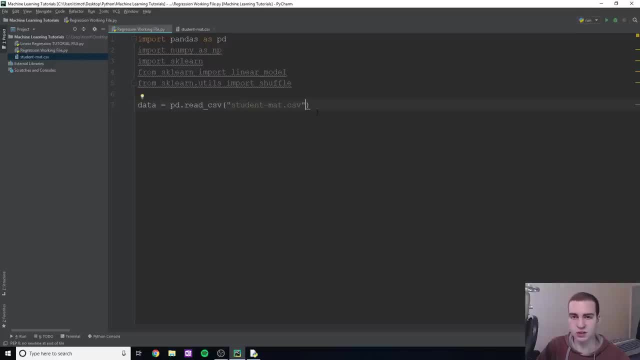 CSV file stands for comma separated values, But to deal with this, we're just gonna have to type sep- equals, and this just stands for separator or delimiter. we're going to do semicolon, Okay, and that's what each attribute is separated by, so that when we read in our data into a pandas data frame- which is what this is actually going to be called here- it gets the correct values, Okay. so now that we've done that, what we're going to do is we're going to set up, we're going to actually trim this data down to what we want it to be or what we need, Okay. 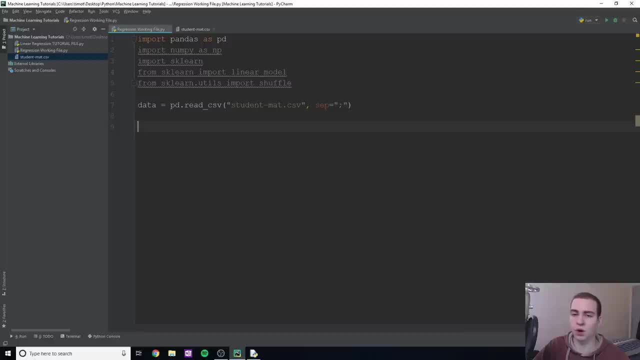 so essentially, you saw we had those 33 attributes. I don't want all those 33 attributes, I only want to use some of them. Now you guys feel free and please- I encourage you- to do this- mess around with the different attributes that you're using. If you want to just test it out, use the same ones as me first, but then add some of your own, remove some, see if you can get your accuracy level up by using different ones. maybe even use them all. you know what I mean. See what you can really do with them. Okay, But essentially what we're going to do here is I'm going to say something called x. actually, no, we're gonna say 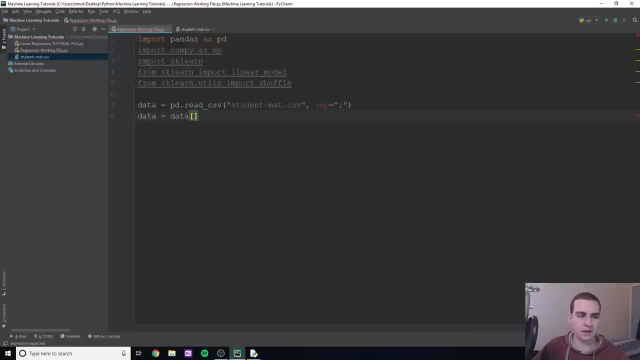 data equals data, Okay, And then in here we're going to put a another little list thing And we're just going to type in the attributes that we actually want. So in this case I'm going to G one, G two, G three. I'm going to do study time, Okay, And what else should we do? Let's say here, study time, And I'm just gonna look at my other screen here See what else we add. Oh, absences and failures, Okay, And these are. you can see the list of 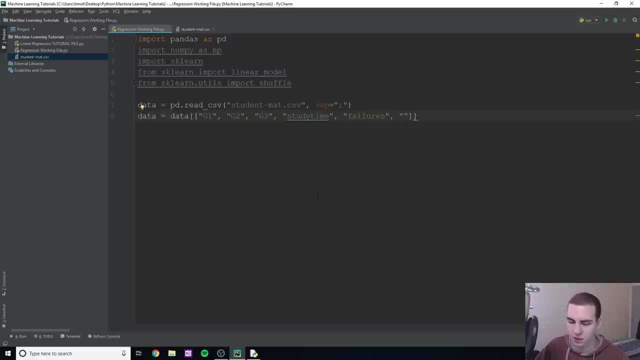 attributes. Obviously, if you go to that website that I was showing you- unfortunately I closed it- And then you can see what all of them actually mean, try to pick ones that only have integer values associated with them, because it'll make your life a bit easier. But if you for some reason pick one that doesn't have an value, integer value, you're going to have to change all the values within this data frame so that their integer, so they can actually work with the thing that we're going to be using. Okay, All right, So these are our attributes, And you know, I'm actually just going to show you what our data frame looks like when we print it out, Because I think it's kind of interesting. So if you do data dot head, this is going to grab the first five elements of our data frame and print them out to the screen and just show us what they look like. So before I change and manipulate the data, I'm just going to print the head out here. So I'll just run this quickly. I already have a configuration set up And you can see that showing us all these different attributes can't show us all of them because there's not enough room in the console- And then what their values actually are equal to. okay, And that's kind of what our data frame looks like. And then, if I want to, I can copy this And we'll paste this down here And you can see what the difference is now with the data frame. Okay, So that's kind of what our data frame looks like. And then, if I want to, I can copy this And we'll paste this down here And you can see what the difference is now with the data frame. And then you can see what the vs button is now And 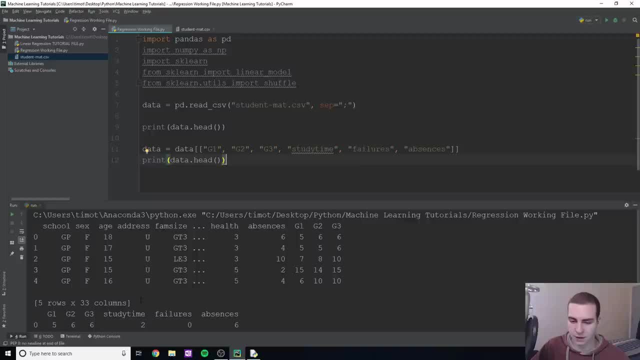 our data frame. Uh, so you can see, we've cut down from five by 33 columns to, uh, it doesn't say: does it? Well, it anyways. uh, we've cut down to however many attributes, this is, which is six. Okay, So now we're going to define what we are trying to predict. So what value? 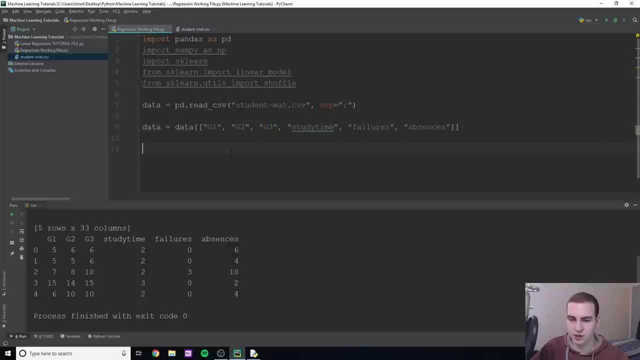 is it that we actually want In this case? we want G three, and G three stands for their final grade. So we're going to predict equals and then, just in this case, we can type the attribute name, which is G three. And this is where I'm now going to go into talking. 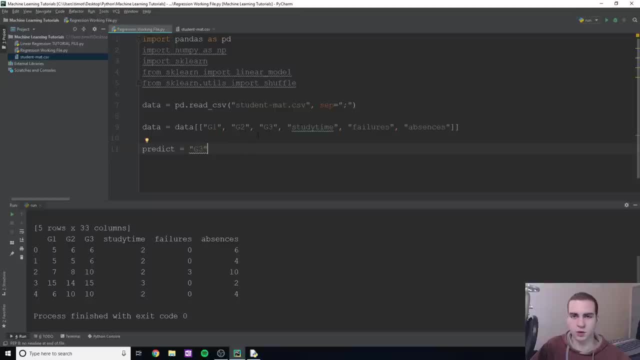 about attributes and labels. See what time we're at: nine minutes. Okay, We'll go for another few minutes before I cut and go to the next video, But essentially, uh, everything here is known as an attribute. right, It's part of a student, Um, and it's unique to. 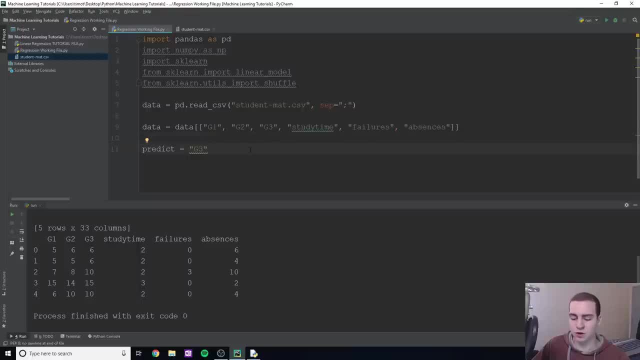 each student like these attributes right, And labels are what we want to um get based on attributes. So in this case, our label is actually going to be known as G three because, based on all these different attributes, we want to determine what G three is now. Yes, 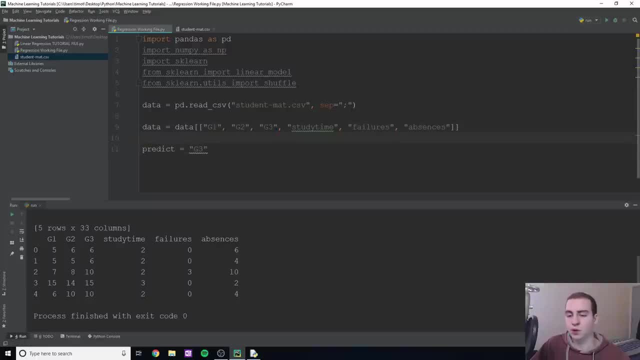 I know I have G three Three in here And it is still an attribute, but we're going to remove that when we um are actually testing and training this data set. Okay, So this uh predict is also known. 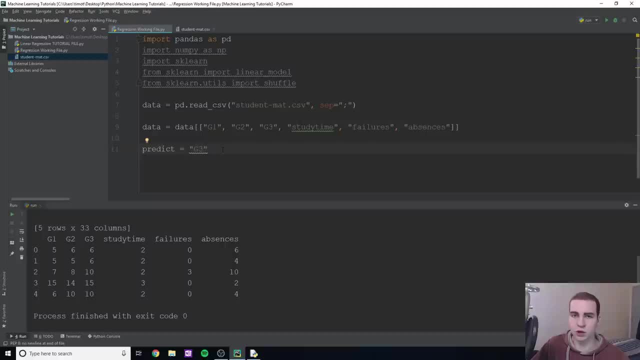 as a label. You may hear people say that, uh, and essentially, label is what you're trying to get right, What you're looking for, And you can have multiple labels and you can predict multiple labels. And you can also predict, uh, what do you call it? You can have, like: 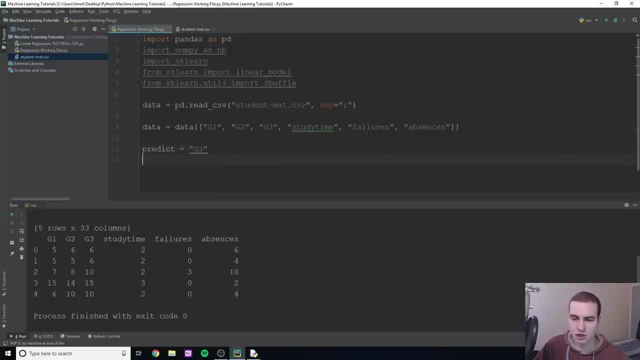 a ton of different attributes. You'd have one attribute: It's: it's a. you can change it around, It's all variable, Okay, So, now that we've done that, what I'm actually going to do is: So I'm going to set up two arrays, and one array is going to define all of our attributes. 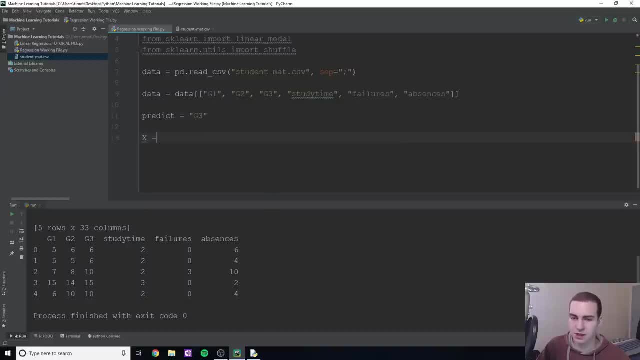 and one is going to be our label, or labels, if we had multiple. So in this case I'm going to say X is equal to, and I think we're going to do MP, dot array. So we're going to set this up in array because this is what we're going to have to use And we're going to actually 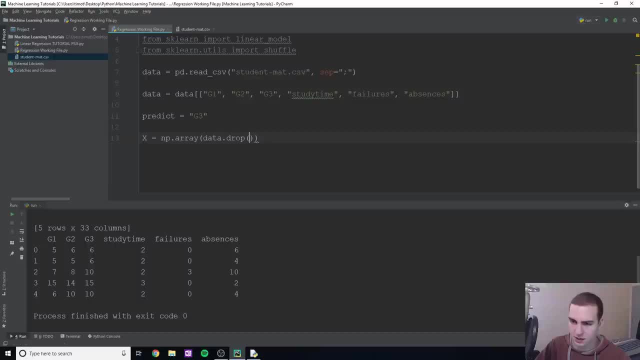 just do data dot, drop, And in this case I think this is what you do for it. At least we're going to drop G three, So essentially what this actually does for us, and actually I need to do this, I think. 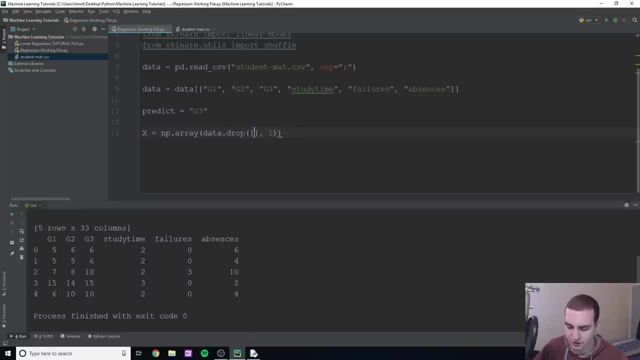 I think, based on what I'm looking at here. so G three, but we'd actually just use predict, So this is more optimized if we're going to change what we're trying to predict, but essentially what we're doing here, right Is? this is going to return to us a new data frame And these 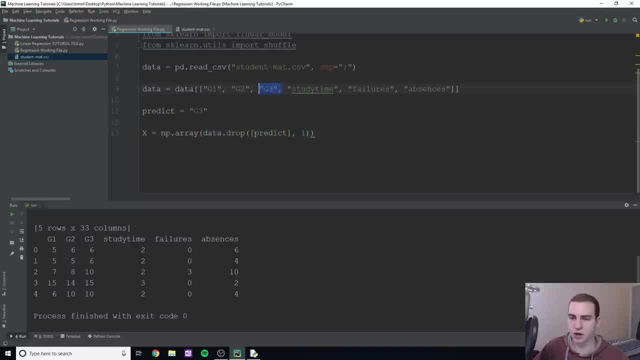 are what these are all called, right, That just doesn't have G three in it, Cause this is going to be all our training data And then, based on that training data, we're going to try to predict like another value, right? Okay, So X and then Y is going to be all of. 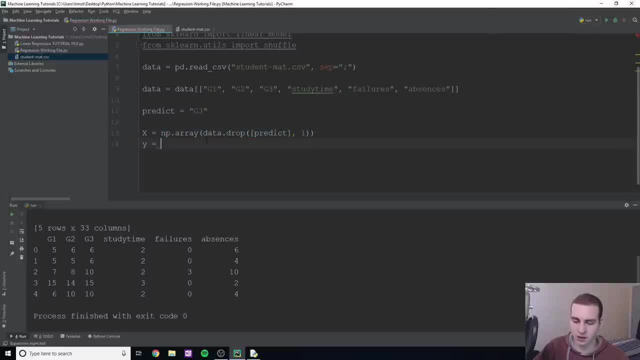 our labels, whereas this is all of our features or attributes. Okay, So what we're going to do now is going to do MP, dot array And then here we're just going to go: data and what we mean for data. We're just going. 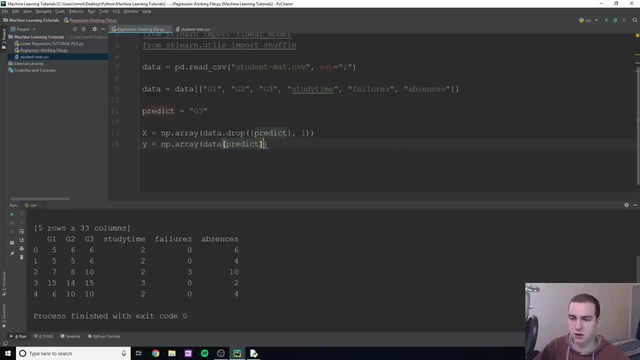 to do data and then predict in here, because we only care about the actual G three value here. Okay, Now let me just check. Yeah, that is correct. Okay, So we're gonna do that- X and Y. Now what we're going to do is we're actually going to split these up into four. 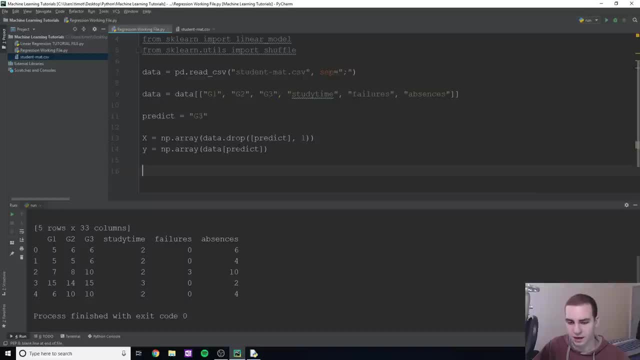 variables. We're going to have X test, Y test, X train and Y train, Okay, And not in that order, but you'll see in a second. So we're gonna do X underscore train, Y underscore train, not equals or greater than sign or whatever that is, And we'll have X underscore test. 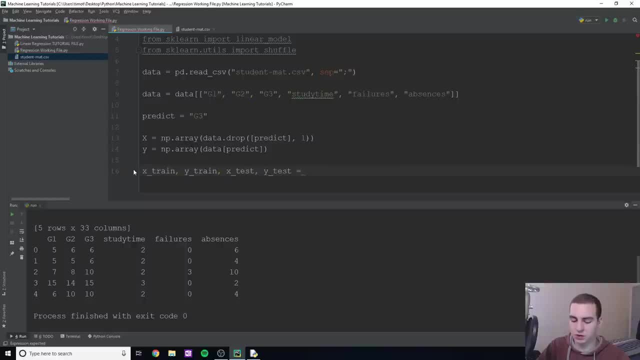 and Y underscore test And this is going to be equal to how? to? what is this command? SK learn dots, linear model or model selection, actually dot train test split. So it's given me all those, which is very nice, And in this case, what we're going to pass, we're going to put in here, we're going to 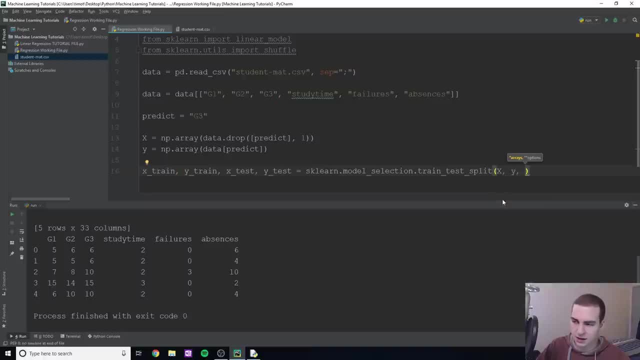 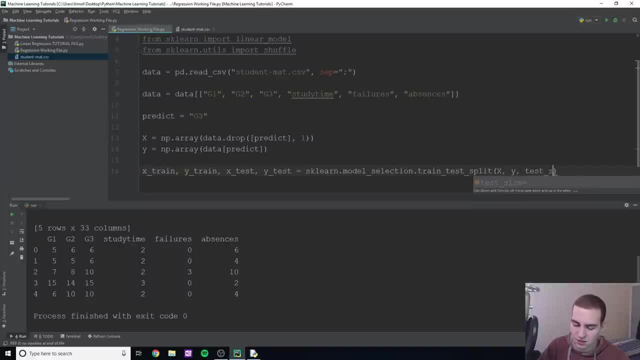 have a look at my other screen test size. This is what it is. Test underscore size is equal to 0.1.. Okay, So let's talk about what this is doing Essentially. We're taking our- uh, all of our attributes and all of our labels, or whatever we're trying to predict and we're 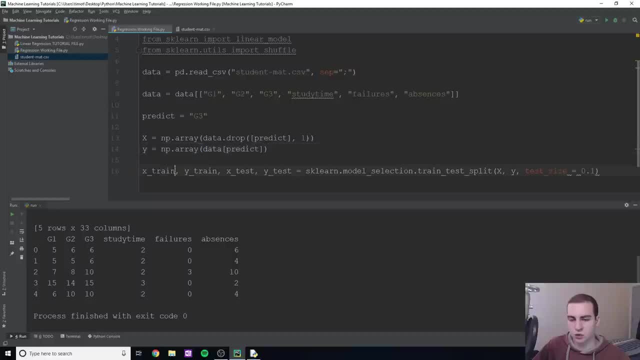 going to split them up now into four different arrays. So we have X train and Y train. Now X train is going to be a section of this array. why train is going to be a section of this array? And then we're going to have these test data. 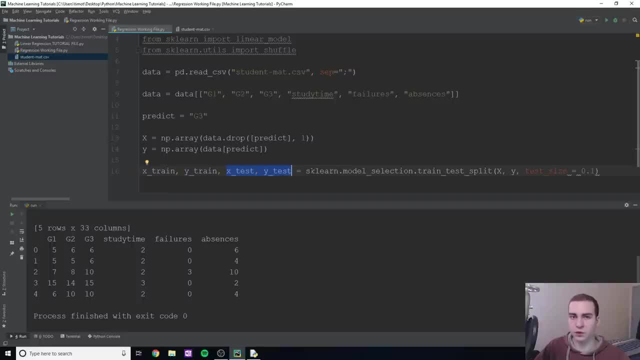 that we're going to use to test the accuracy of our model that we're going to create, or of our algorithm. All right Now. the way this works essentially is because if we trained the model off of every single bit of data that we have, 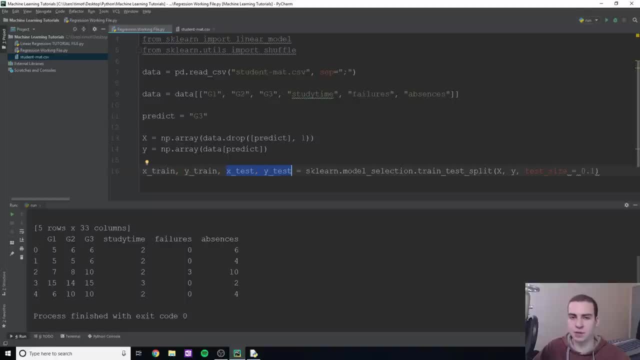 and then it would simply just memorize patterns, right, Because computers can memorize things like amazingly. So think about it kind of in a way, say like you're in class, right, And actually that's a bad example. Let's just say this, right. 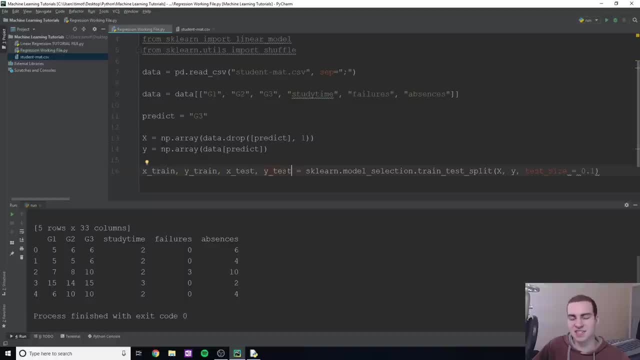 If we train the model off of the data we're going to test it on, it's already seen that information, So it already knows what the answer to that question is or to that prediction. So we can't train the model off of our testing data. 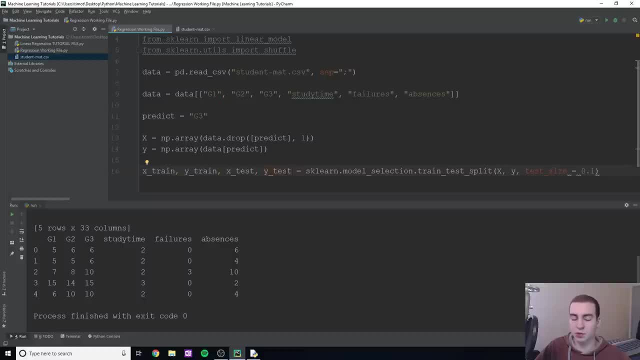 Otherwise we're going to get inaccurate results, because it's going to be able to pretty well get perfect because it's already seen that information. So essentially what this does is we're splitting up 10% of our data into test samples so that when we test, we can test off of that. 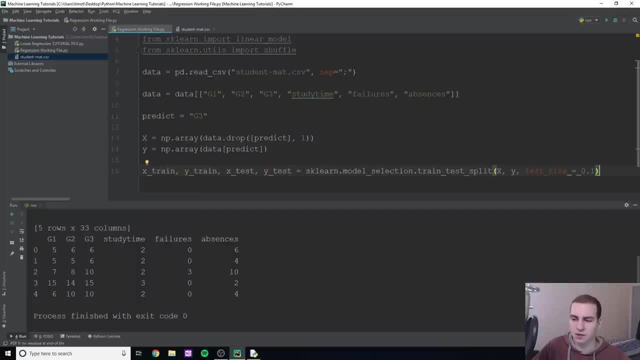 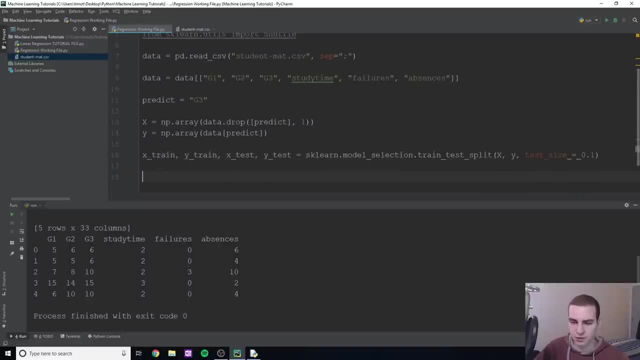 and it's never seen that information before. Hope that makes sense to you. And this is just what this whole mess of code is doing for us. All right, Test size and the X and Y is just taking our labels and features or attributes or whatever. Okay, 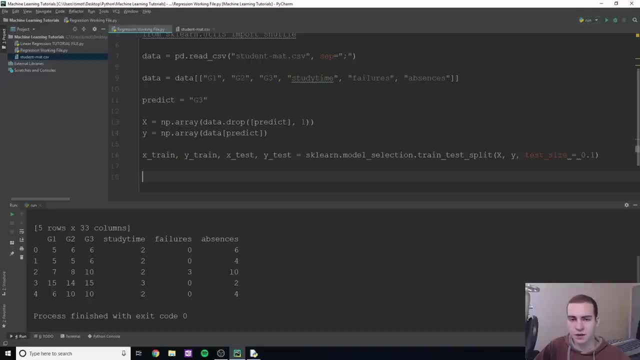 And I think I'm actually going to cut the video here. In the next video we're going to go into actually applying this into an algorithm, talking about how that algorithm works mathematically, And then maybe I'm not sure if it'll be in the next video. 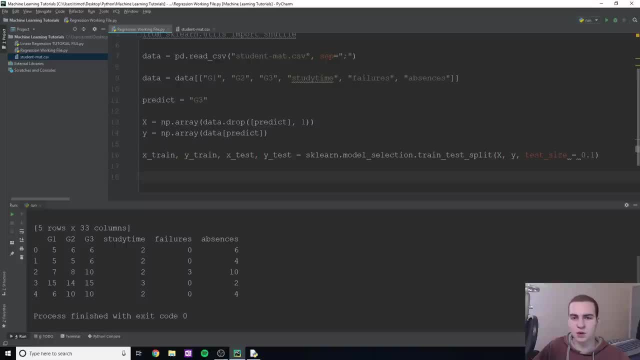 The one after that will do predictions and so on. with that, Okay. So if you guys enjoyed the video, please make sure you leave a like and subscribe, And if you want exclusive updates on when the next machine learning videos are coming up, make sure to follow my Twitter. Tech with Tim. 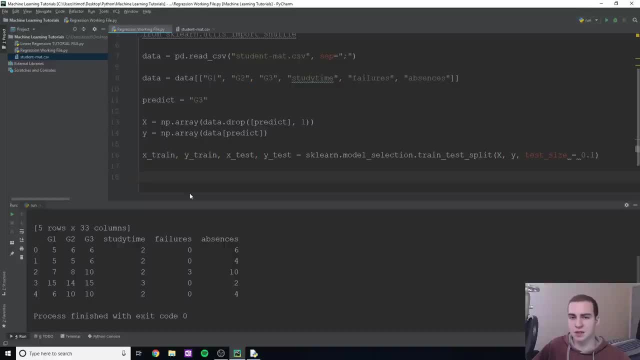 because for me posting pretty much all the information for this. Anyways, I'll see you guys in the next video.